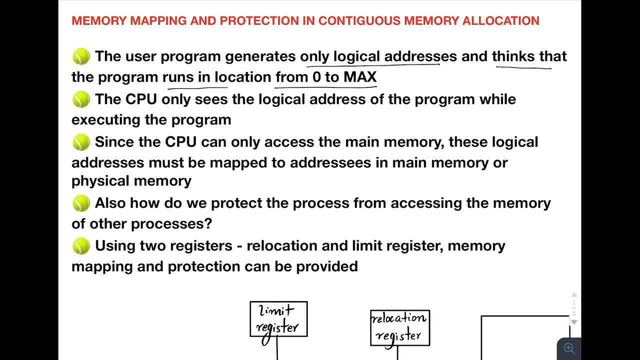 kernel sees the programs differently, right, so we will look at that later. and the CPU. right, it only sees the logical address of the program while executing the program. right, so CPU only gets the password. so it starts from the program counter. right any program, it will see the program counter and start executing. 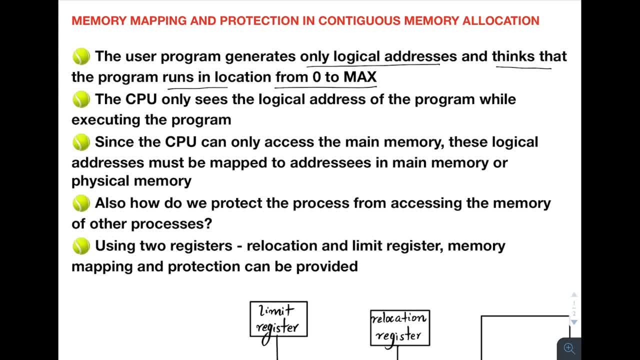 right and in the program counter the logical address of the program is stored right. so the CPU only looks at the logical address space of the program, not at the physical address space. but since the CPU can only access the main memory, this logical address must be mapped to addresses in the main memory or physical 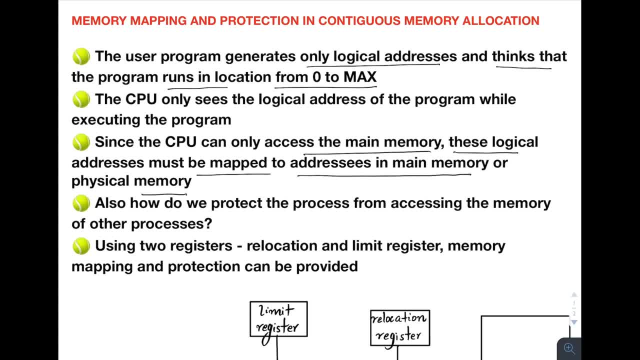 memory. we already know that CPU cannot access the hard disk right directly, right. so it can only access some cache and then the main memory or the RAM directly. but CPU here is only seeing the logical address, right, but the memory it can access it is a physical memory, right? so therefore you. 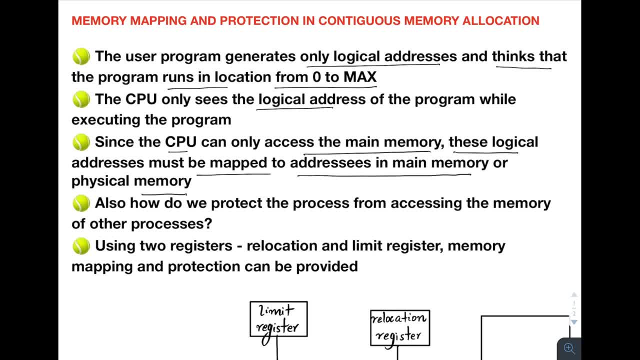 have to convert this logical address to the physical address? right, then only the CPU will be able to fetch, or I mean write, instructions with the RAM. right. and also, how do we protect the process from accessing the memory of other process? right, this also we have to take care of. right, the kernel has to take care and it. 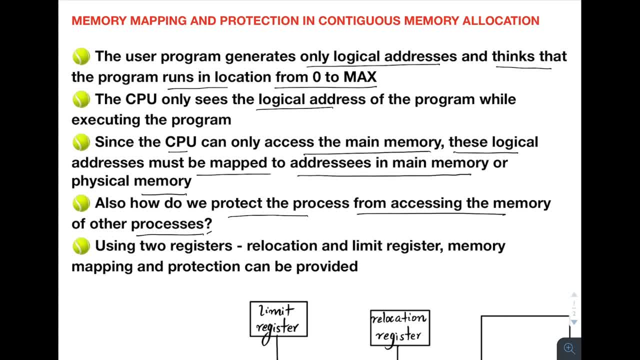 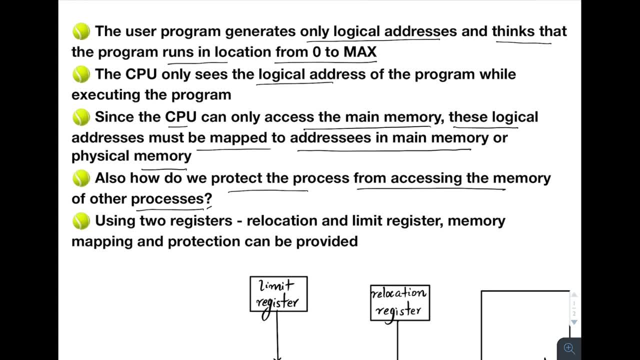 has to prevent one process from accessing the memory of the other process. right? so how the? I mean how we can achieve these two goals of memory mapping from logical to physical and also providing memory protection. so this we can do with using two registers: relocation register and limit register. that means we need to take the help of the 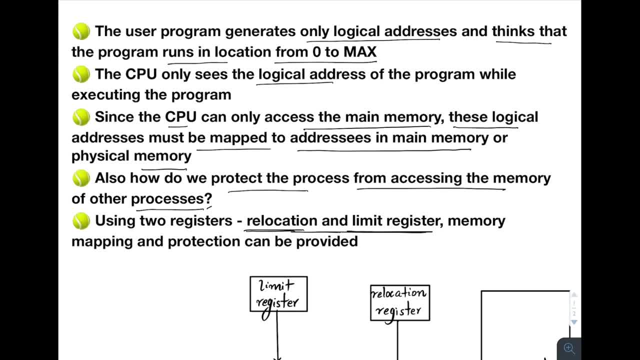 hardware. so because these registers are the part of the hardware, right, so we need to take- I mean help from them- these registers. then we can provide the memory mapping and the protection. so we will see how we can provide this. then we can use 2 registers different. are reichters, then we can provide the memory mapping and the protection. so we will see how we can provide this. might we want one? so we need to be asked as to this. you know, the memory map, this is for setting the horrific relimiting Matt. so then it is also we uncle jar is. 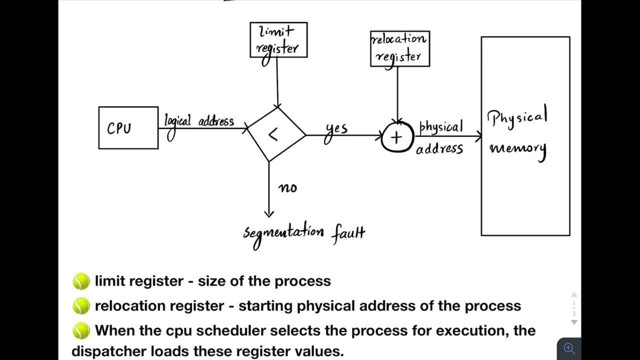 available in our machine. then the похive T Nav, the a, and here you need to note the textiles there above schönOUGH and manuscript or any democraticERT that knowledge which is eraser I in the commercial case. so you have two registers, limit register and the relocation register. so limit register is the size. 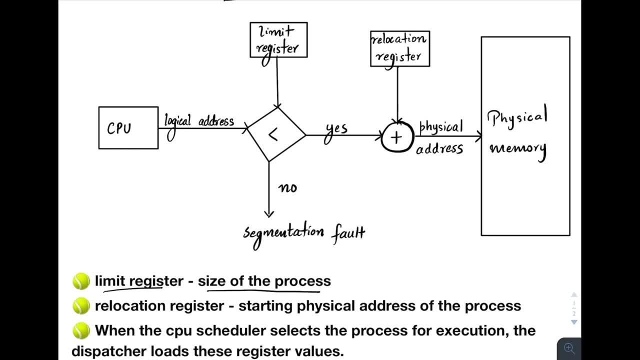 of the process. so this in this. so there will be two registers, right? so one will be limit register and one will be the relocation register, right? so in the limit register, the, the size of, i mean the value stored, will be the size of the process, or also you can tell this as the range of logical 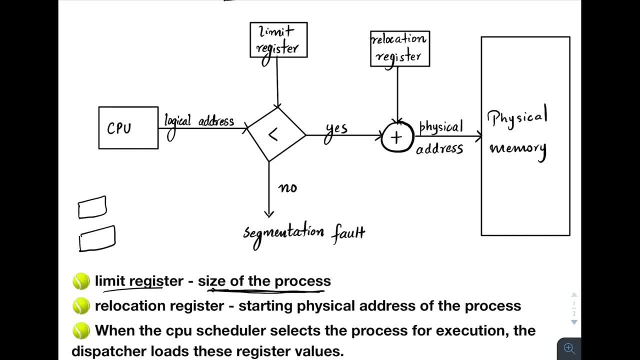 address that the process can take, right. so that means: see this. let's say- i will take example here- let's say: this is a process right from zero to max, right? so the maximum logical address that this process can take is max, right? therefore, max will be stored in this limit register. so this max is 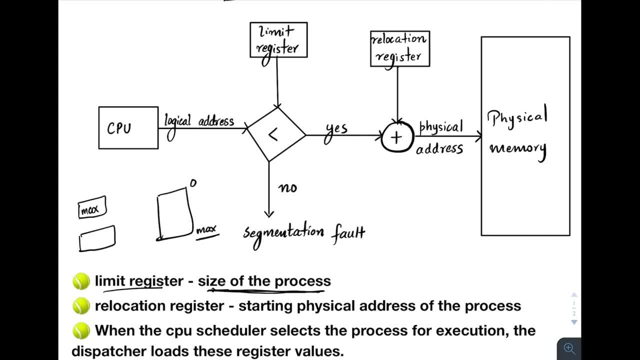 the size of the process. basically, right now, what is relocation register? so relocation register- this is sometimes also called as base register. so relocation register means that, okay, this address can change, right? i mean, while the program is running this, uh, relocation register address can change. that's why the name relocation, right, this is the starting physical address of the 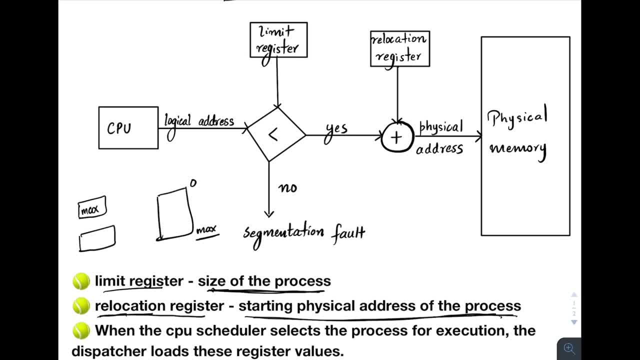 process right. so this is normally given, provided by the kernel. so the kernel initially will i mean provide a initial start address to this process right? and we already know that this is a contiguous memory allocation right. that means, let's say, and this is the physical memory right. 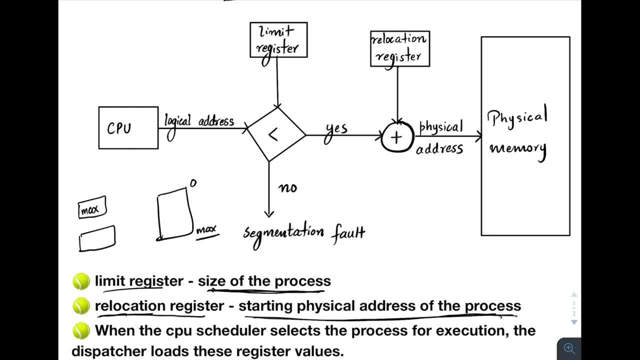 so, let's say, kernel decides that, okay, this process will, uh, start from here, right, i mean here- to here, right, so it is, there is some, is some address x and this is, let's say, x plus max, right? so this x is actually, this x is actually the relocation. i mean, this x value will be stored. 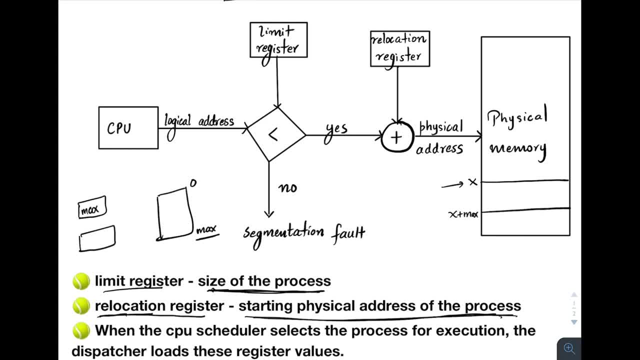 in the relocation register and this is decided by the kernel. so the kernel will decide that, okay, this is the continuous memory allocation technique. so i will allocate- i mean i will allocate this process right right- some p from x to x plus max, right in the physical memory, right here. 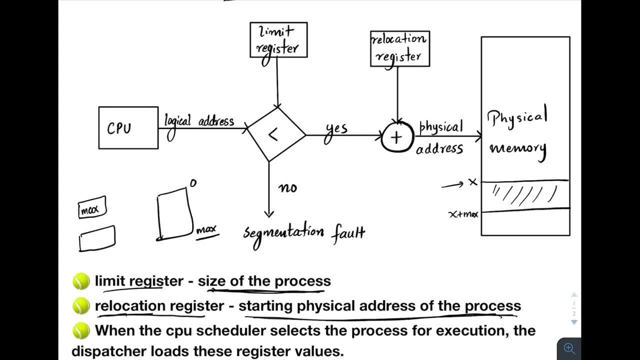 so this x will be the relocation register. value and limit register with value will be max, right, so this x from x to x plus max, this process will be there right in the memory. so this limit register contains the size of the process. so this will be max. now let's look at how this, and also uh. 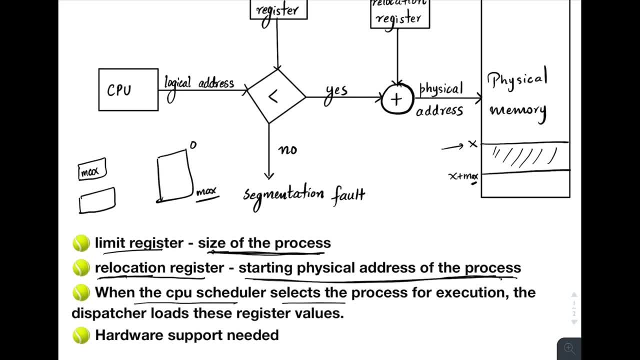 i forgot one more point. when the cpu scheduler selects the process for execution- right, so we know the cpu scheduling is done, right, there are many algorithms for it, right? so once the cpu had decided- i mean cpu algorithm- had decided: okay, this process now needs to be settled on the cpu. 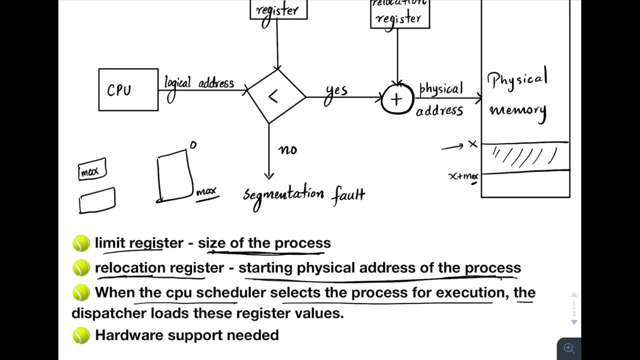 then there's a dispatcher, right. so this dispatcher, what it will do, is it will load the these register values, right, this uh, two register value, the register and relocation register, as well as the limit register value. it will load these values from the pcb of the process, right, and this is the? 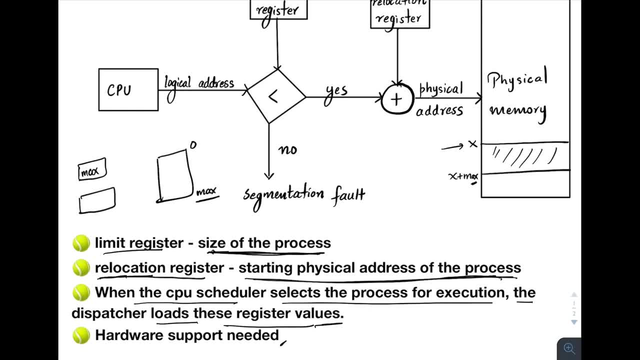 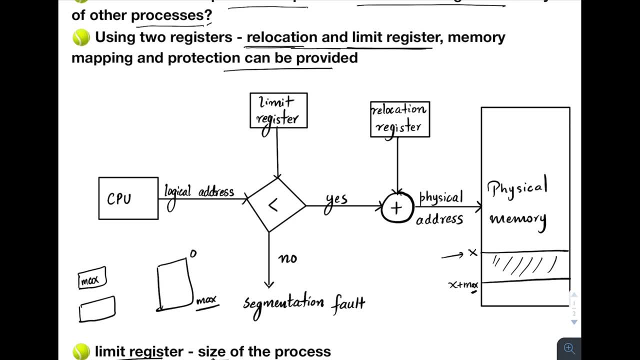 part of the context switch. actually, i told that in this case, hardware support is needed. now let's look at this diagram and understand the whole concept. so you have the cpu right. it will generate the logical address from zero to max, right, and since the address is starting from zero, you don't, i mean, you only need to check. 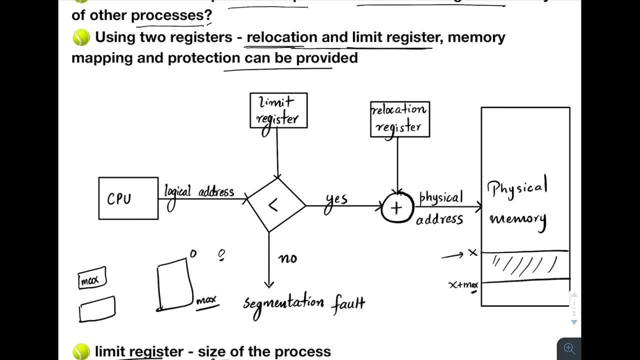 whether. see, we also need to provide the protection here right. so for this we need to check if the- i mean the in the limit register- the max value is stored right. so if the process is starting from, it means it is trying to access the memory location of some other process, right? that's why we are 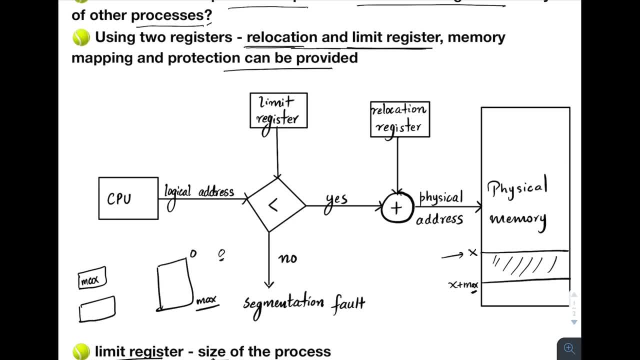 checking here, right? so if the logical address is lesser than the limit register, right, that means, that means it is trying to access its own memory, right? but let's say, if it is greater than the, i mean the limit register, right. so in this case what happens? basically it is trying to access. 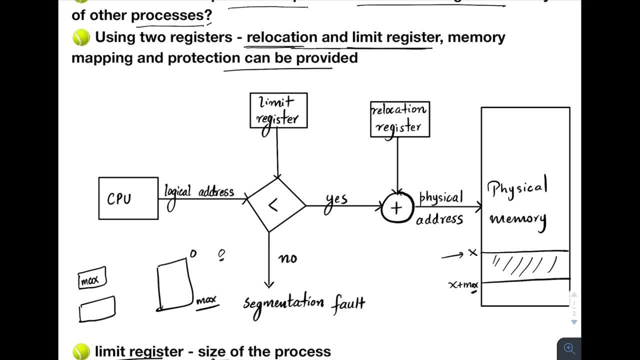 the memory of some other. so it was zero to max, right. but what if it is trying to access max plus one, right? so what if the logical address is max plus one? that means it is trying to access the memory of some other process, right? so in this case a segmentation fault is generated, right? 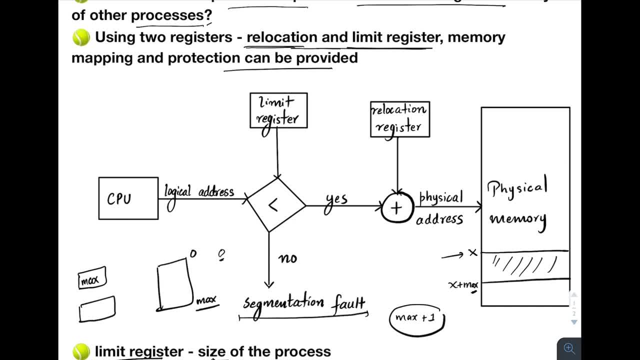 so basically, i mean interrupt will be generated on the cpu and then the kernel will send a signal to the- i mean to the program- and then basically program will be terminated by default. so this is the signal that is sent: segmentation fault by the kernel. now let's say: 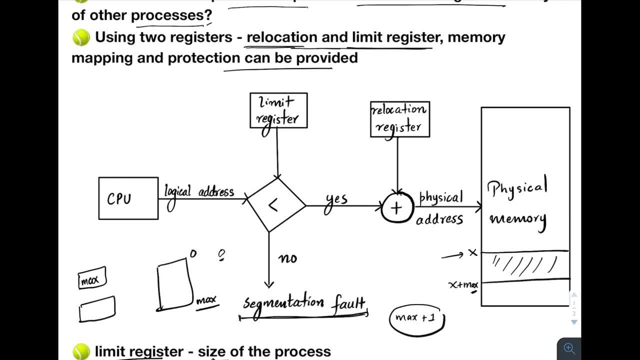 the value of logical address is lesser than the limit register. so in this case, what happens now? so now we have provided the protection right, but we also need to provide the mapping. so for mapping what we do, so we already have the relocation register right that contains the 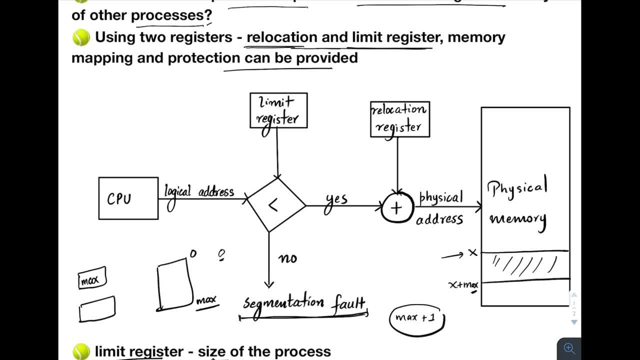 starting address in the physical memory. now, if, if you sum this relocation register with the logical address, right, so you are going to get the actual physical address of that instruction, right. so that's what we have done here. so if you see, the relocation register is sum of with the logical address. 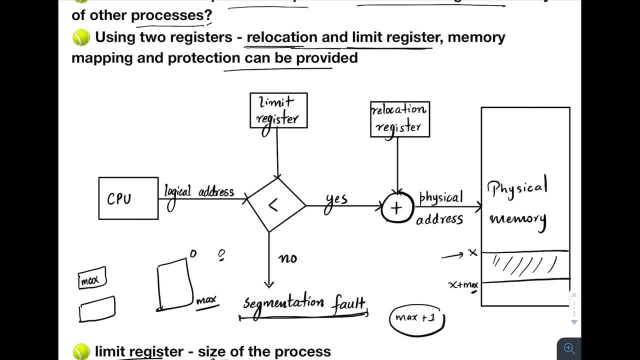 and we sum this up: you, you are you, i mean you, i mean the mapping is so the mapping for logical address, physical address, is done. i mean we can take an example to understand this. so let's take an example to understand this, how this is done. so i'm just taking example. 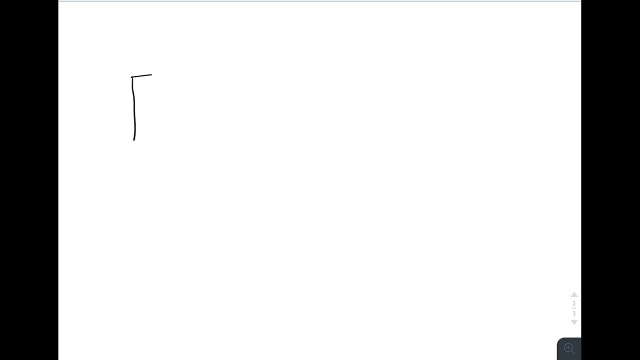 of the mapping part, right. so let's say: this is the process, right. and let's say: there are many bytes of instruction, right, there are many bytes here. let's take the example zero, one, two, three, four, five, six, seven. let's say right. and now let's say: uh, now you have cpu here. 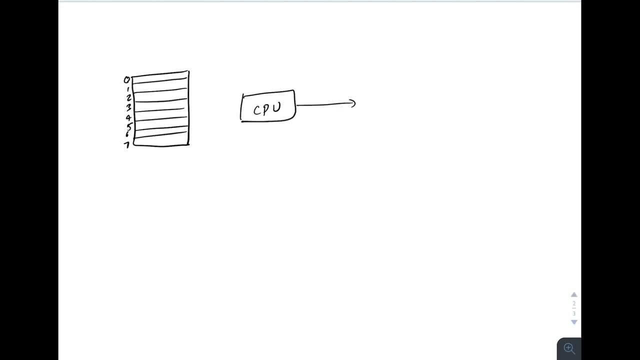 and cpu is currently, let's say, executing the uh logical address. let's say this one, second, right. so cpu sees this second and logical address right now, let's say initially, when the program would have the kernel would have already load, already provided a value for the relocation register, right relocation register. this will be ram here. 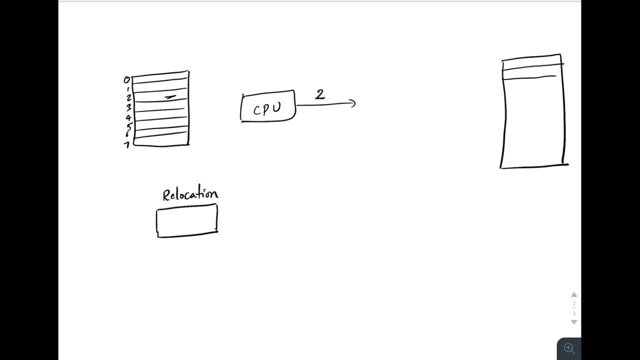 and ram, also with, let's say, it's divided, it's a divided byte by byte. let's say zero, one, two, three, four, five, six, seven, eight. right now, let's say, um, the kernel assigned a value. let's say, uh, let's say this space was free and this is signed, this value. 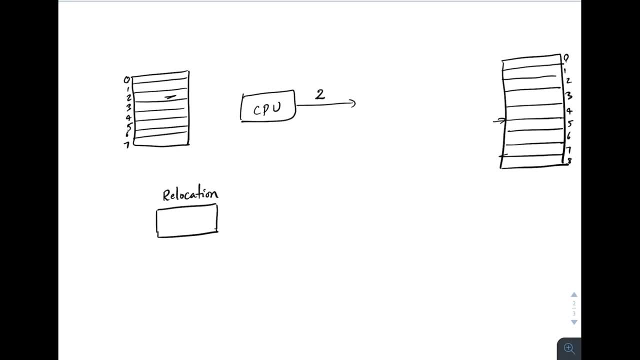 five, let's say: right, so this is five here. right, so it is signed five here. so this is the work of the kernel to assign the relocation register value. right, because the kernel has to decide where the, where there is some continuous space free in the main memory, and then we will give you this right. 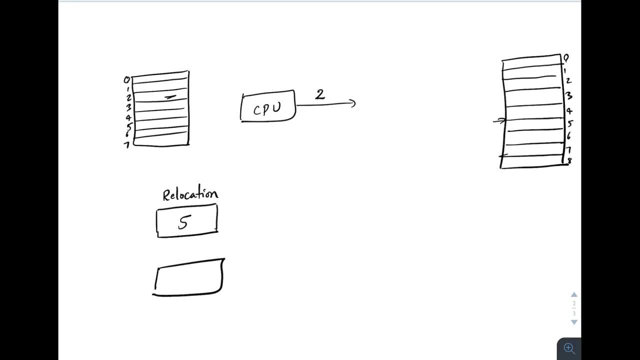 and what is the value of the- um sorry, the limit register here? that is the size of the process. what is the size of this process if you see one, two, three, four, five, six, seven, eight, eight bytes, right? so eight is the limit here, right? so let's uh think that the protection is done, right you? 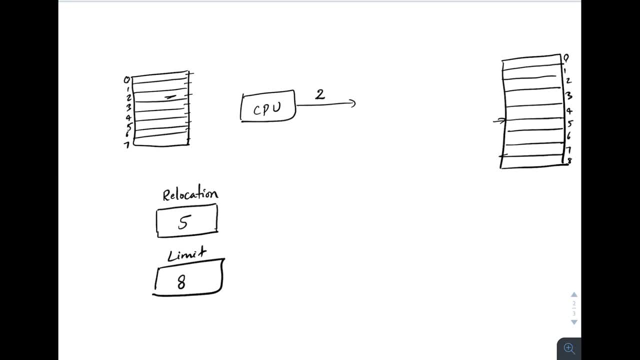 have checked right this, uh. now we are at two right. two is lesser than eight right. that means it is trying to access its own memory right now. it will sum this up: right, so we already know that this process is starting from five right, but we have to uh. 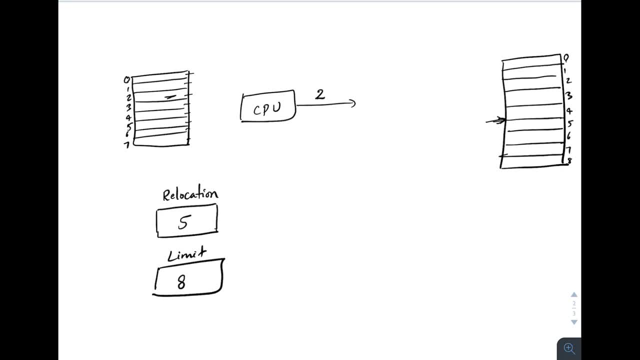 so add, add this five. so basically, if you see, if you put the process here right, this process here here, uh, okay, let's okay. if you, i mean if you start from five, what will happen is: this process requires eight bytes, right? so five plus eight will be 13, right? so this cannot happen. 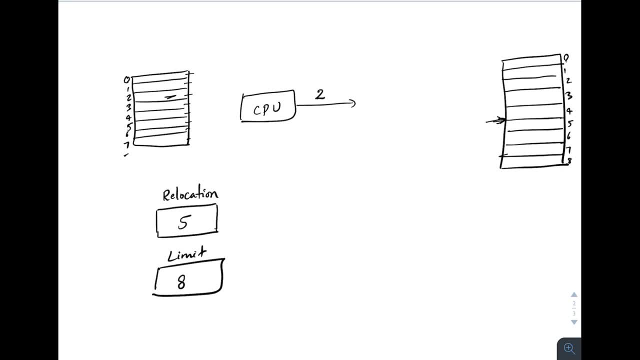 because ram is only of nine bytes. so what we can do is we can start this from, let's say from here itself. let's say from zero itself. let's say so basically, here relocation was zero. let's say it's starting from zero itself. right? so the kernel assigned this. 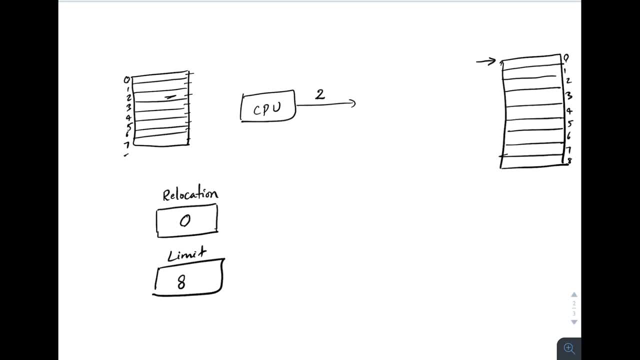 as the relocation address zero, right, that means process will start from here. now, what you can see, this is a continuous space, right? you can put the process here. so this is a logical address which will be mapped to here. i am putting it here because from so, basically what will happen is this: 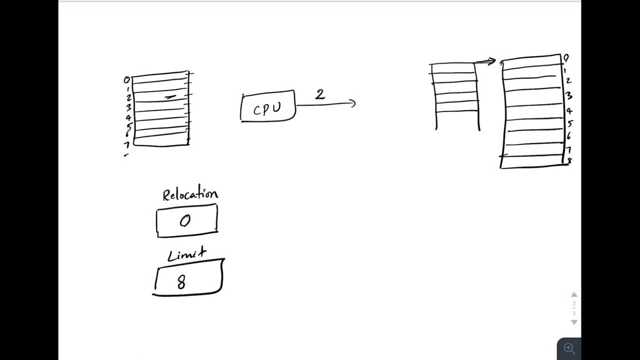 uh, let me divide this process. so this is a logical address space. basically, this will be mapped to this right. this will be mapped to this. this will be mapped to this right. this will happen. so this, this mapping, will be done. this is logical address and this is physical address. 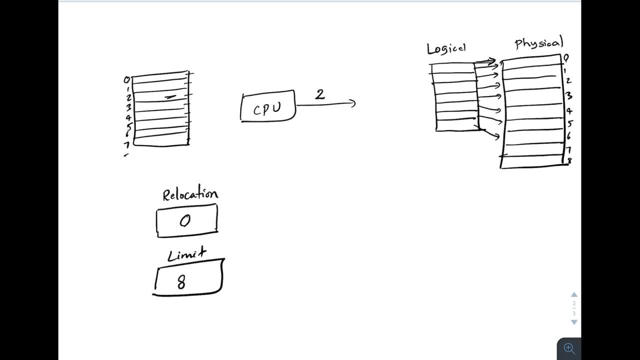 and what is the base address? so base address or relocation, was the zero, so that means the zero i'm. the zeroth byte of this physical address will be mapped to the zeroth byte of this physical, sorry zeroth byte of this logical zero. one, two, three, four, five, six. we'll continue this seven also. 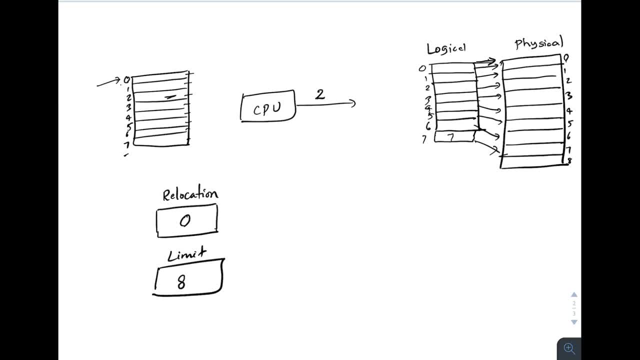 this will be mapped here somewhere. so basically, zeroth address of this, zeroth logical address will be mapped to the zeroth physical address here and first logical address will be mapped to the- i mean the first physical address, first byte. so here we have taken the reference as zero. 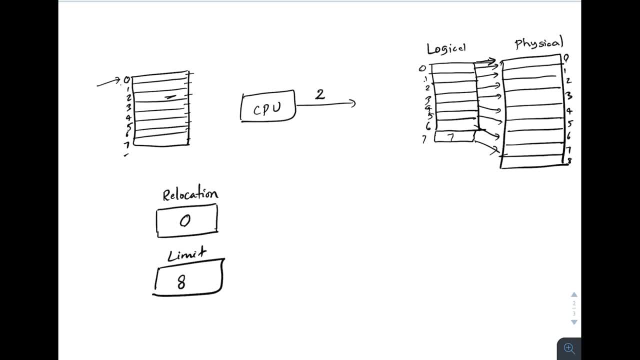 so both are same. but you can also take another example where it, let's say, the relocation was one, right, then i mean, let's take that example. so in this case, what will happen? right? basically, what we will do is you will sum this up right. so for mapping this two, we will sum this with the. 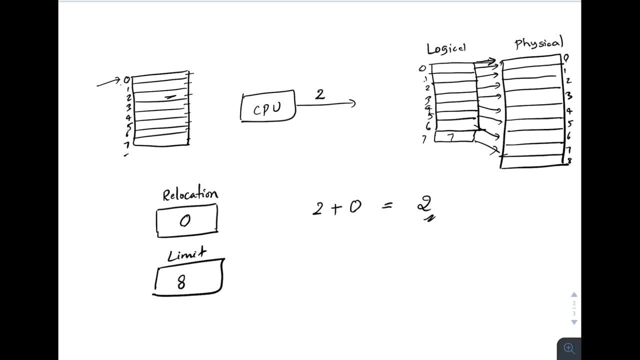 relocation register. two plus zero, you will arrive at two. so this two is the, so in this case i mean the physical and logical address are same. two is mapped to two, so three plus zero will be mapped to three in the physical right. but let's take the example. if this is a logical address, let's say so. 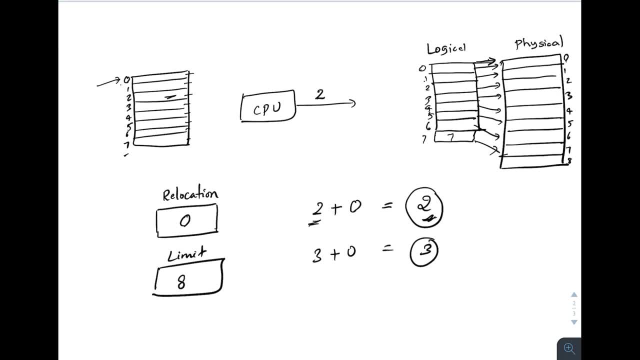 this was not the case. I will just remove this. mappings- Sorry. Let's take this example. What if 0 was mapped to 1, right, That means relocation was 1, not 0, right. So in this case, what will? 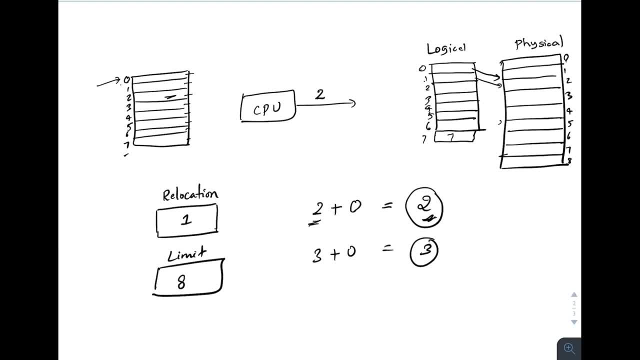 happen, 0 will be mapped to 1,, 1 will be mapped to 2, right, Similarly, everything will be mapped. So in this case, if you see, the relocation register has changed. So you will again sum it. 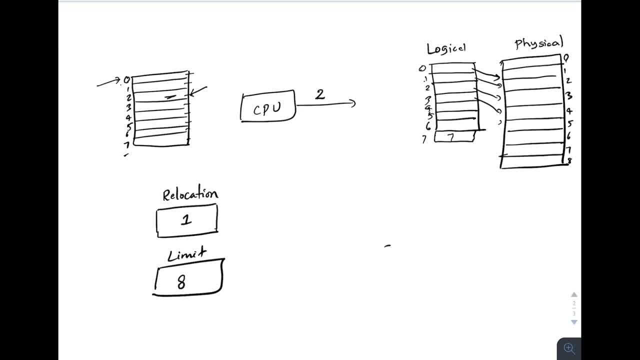 up. So for the second byte of this logical address, we will sum 2 plus relocation register. you will arrive at 3, right, That is what happens. This second byte of the logical address, if you see, is mapped to the third byte in the physical address, right? So similarly, for third byte in 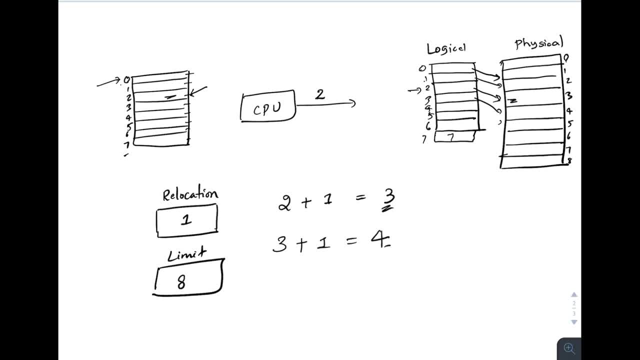 logical address plus 1, really fourth byte in physical address, right? So this is the fourth byte. This will be mapped to fifth byte here, right? So same thing will happen, And I hope you would have understood how this mapping is happening, right? 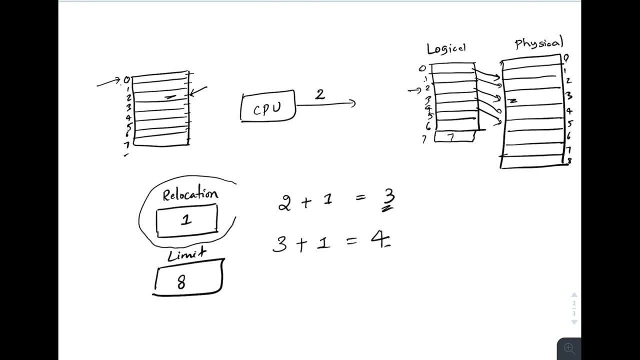 So this relocation value, so what is the initial starting address of the process in the main memory or physical memory, will be assigned by the kernel And then limit register is the size of this process. Here we have 8 bytes. size of the process, 8 bytes. So limit is 8.. Now you just